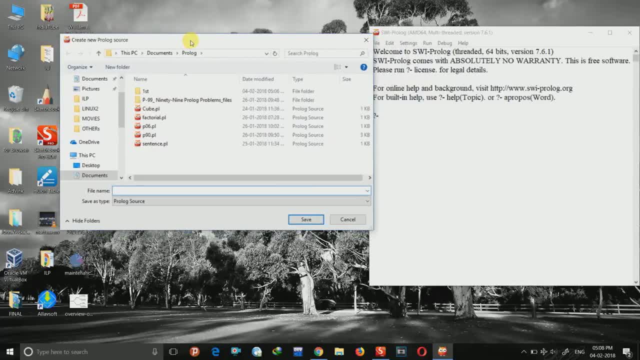 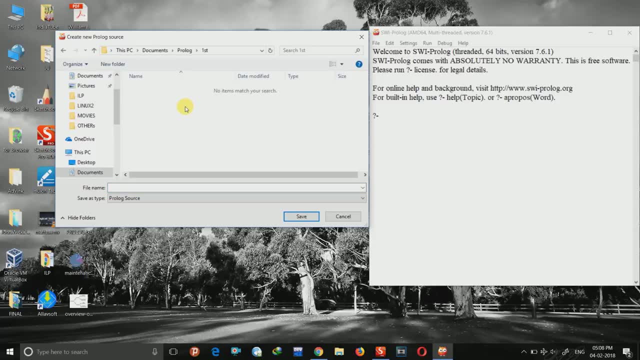 Now you can see that you will be presented with the location and wherever you want to save it. save it. Okay, I just want to save it here and while writing the file name, you see that save as type prologue. source is written over here. 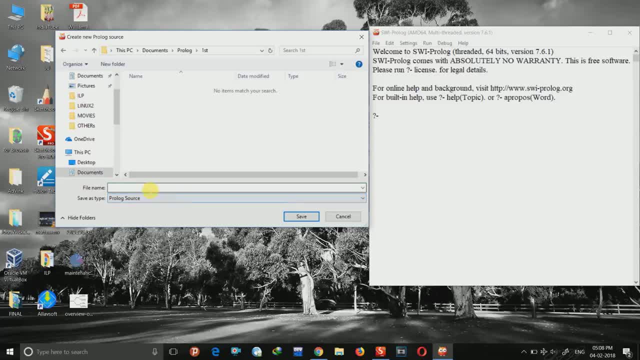 And if not, then select it Prologue source And then click on save. Now you can write any random file name, So let us just write facts, because we will be writing the code taking the facts, So it will be meaningful. Factspl. You will include this extensionpl. Okay, 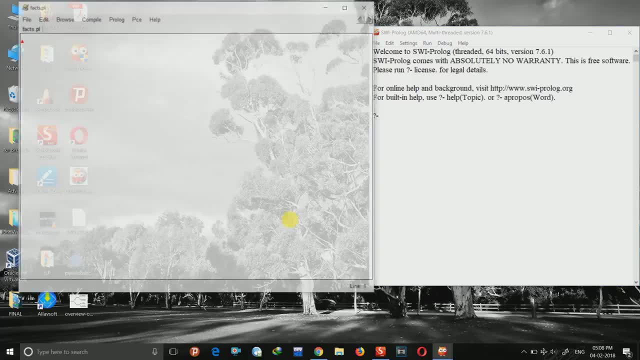 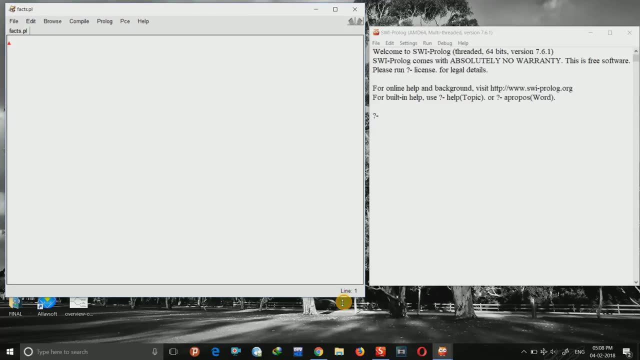 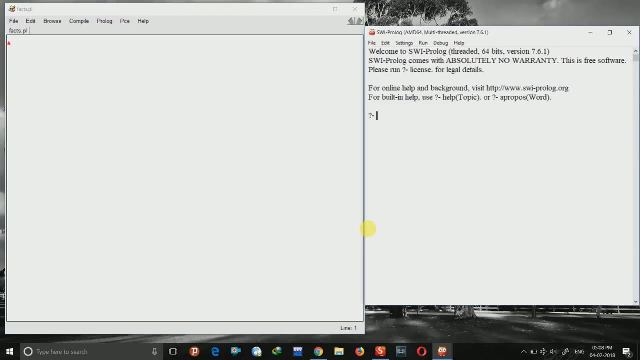 And then click on save. When you click on save, then you can see that the editor will open. This is a prologue editor. Okay, Now I will just maintain its size So we can start writing our code. So I had shown you in the previous lecture what are facts and how to write a fact. 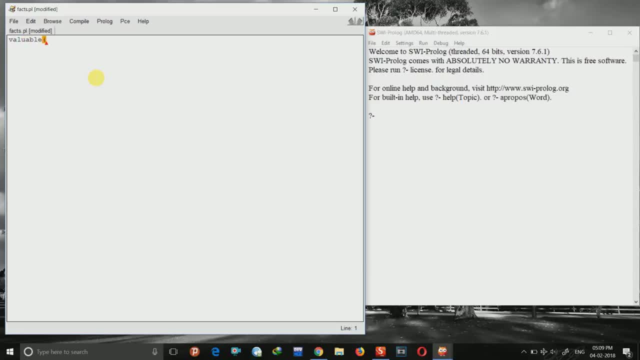 So let us include a fact, Like we include valuable gold, Okay. And then, after writing a fact, after writing any number of facts, Okay, When you are done, you need to compile it. So click on the compile and then compile buffer. 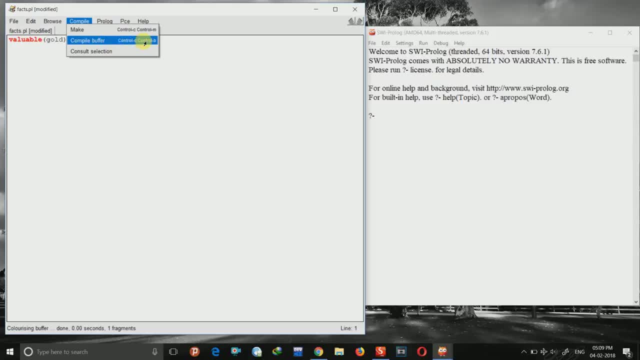 There is also a shortcut: Press c and then control b. Okay, Click on okay And it will be compiled. Now in our query section you can post a question like valuable gold? That means, and then full stop. That means: is gold valuable? 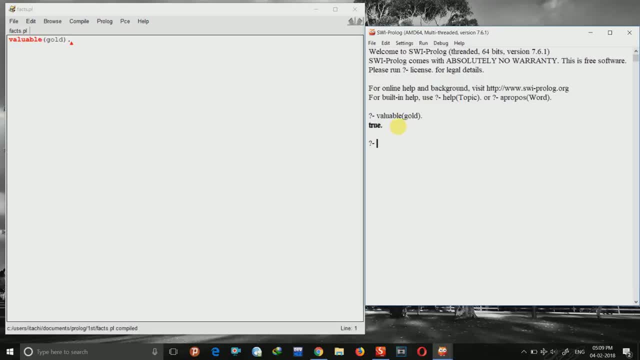 Press enter, Then it is returning true because gold is valuable according to our database. This valuable gold is our knowledge base. Okay, So what we have written over here in this code section is our knowledge base, And this is the query section where we ask the question from the prologue machine. 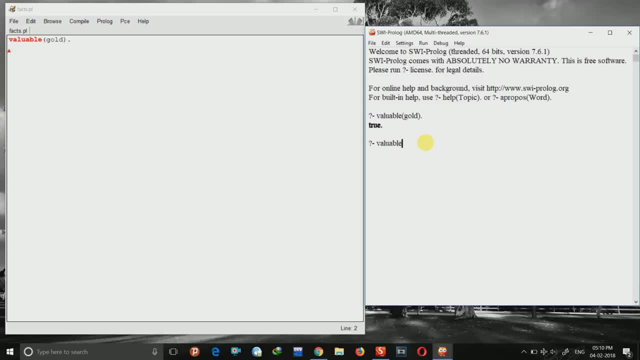 Okay, Now suppose we ask a different question, like valuable salt. So since salt is not in our database, So since valuable is in our database. So while comparison it will find, it will find that valuable relationship exists, But while comparing its parameter, like gold, 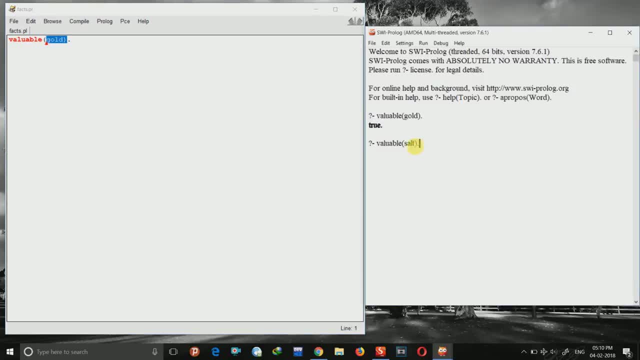 When gold is compared against salt, then it will not match. Okay, So it should return false. So you can see that it is returning false. Okay, So let us quickly add some more facts. Now suppose we have included all these facts, Okay? 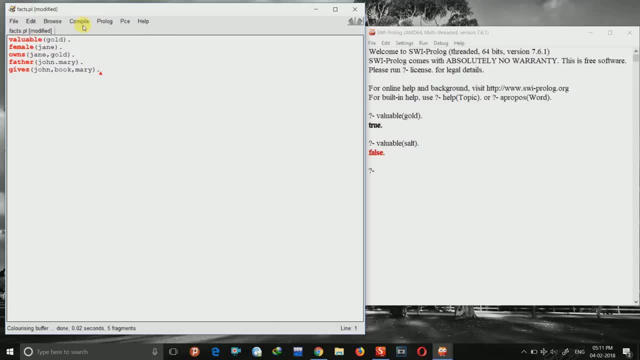 So we need to compile it. You can compile it from here or use the shortcut buttons Control c and then control b. So it has been compiled. Okay, So you can see here that it has been compiled. This is returned. This is written. 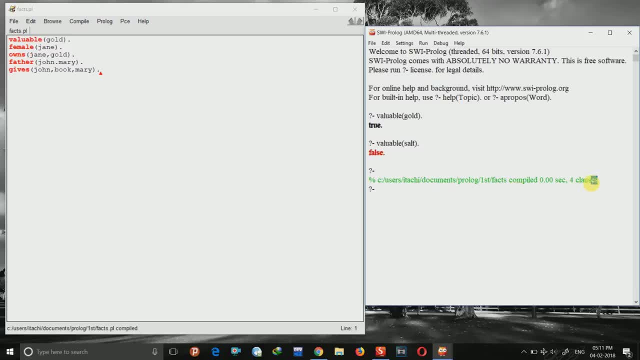 And four clauses. Four clauses have been compiled, because one was compiled earlier. You can see that here there are five clauses. So after that, suppose we post a question like father, marry comma, Marry comma, Jane, Then full stop. Then what should the prologue machine do? 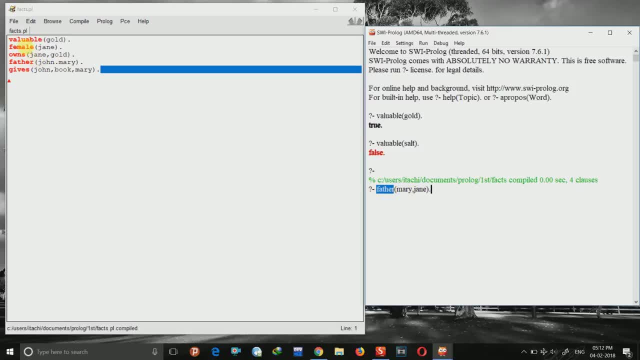 It will search for this relationship father. So you can see that we have only one relationship Relationship with the name father, And in here it is written John dot marry. Actually it will be John comma marry. So let us see This is a returning error, because the relationship father 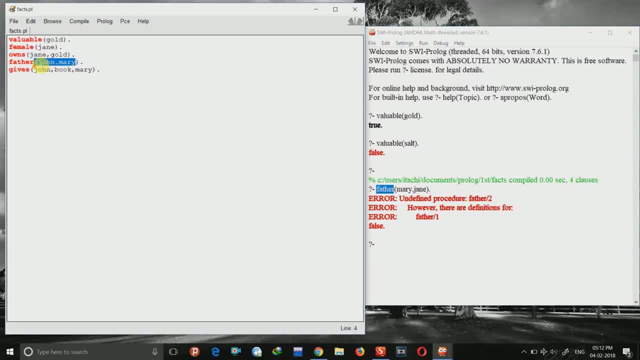 We have defined only one parameter because our separator was comma, But by mistake I have included in here dot. So it is telling us that whatever question we have posted is of parameter of length two. So father slash two. But however, there are definitions for father slash one. 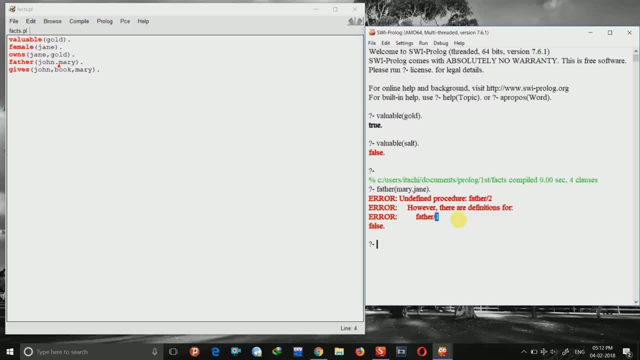 That means the relationship which we have defined in our knowledge base is having only one parameter, And we are asking that relationship with two parameters, So it will return an error, Okay, So let us quickly modify it and see So in here there will be comma. 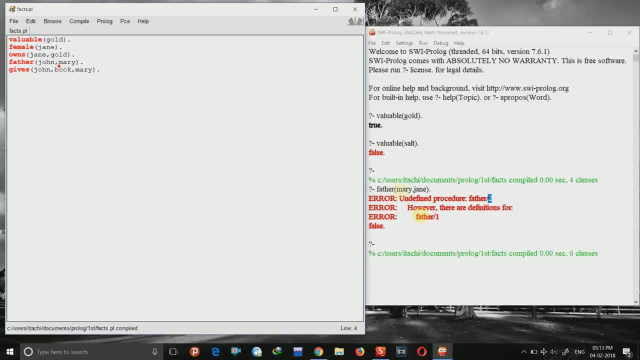 Control C, Then control B, Then okay, Let us now ask the same question. Okay, Father, marry, comma Jane. Now you can see that father. Here there is father. Okay, We have two parameters: John comma marry. Here we have two parameters: marry, comma John.